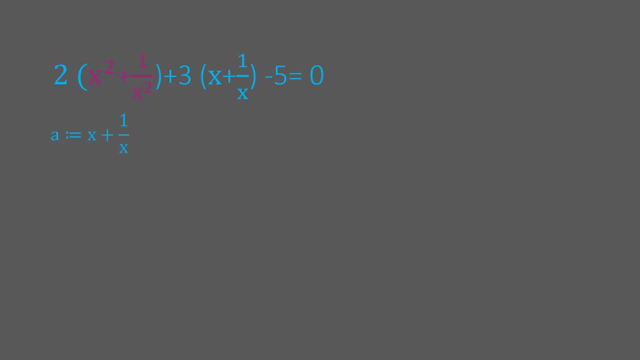 So, in order to get rid of this term, we have to square a and a square. After adding the two to the left side of the equation, we get this result. Substituting this, you get an quadratic equation. You can solve this, for example, with the quadratic formula. 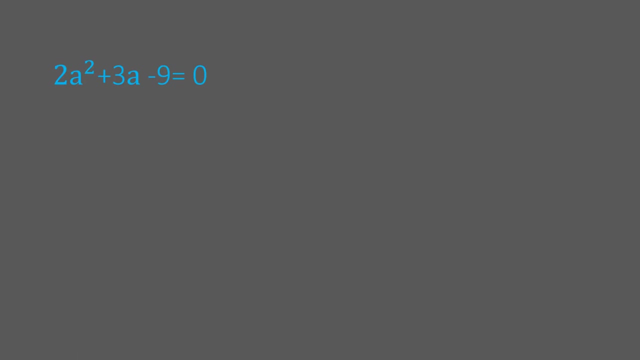 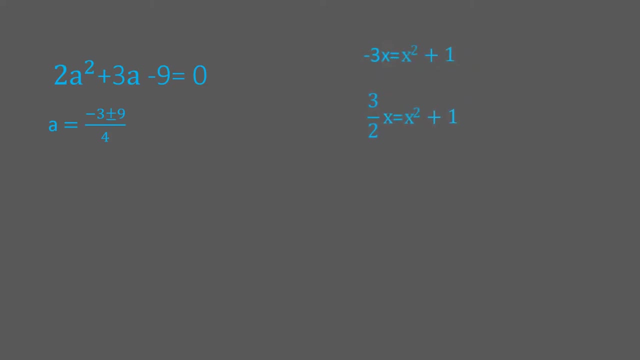 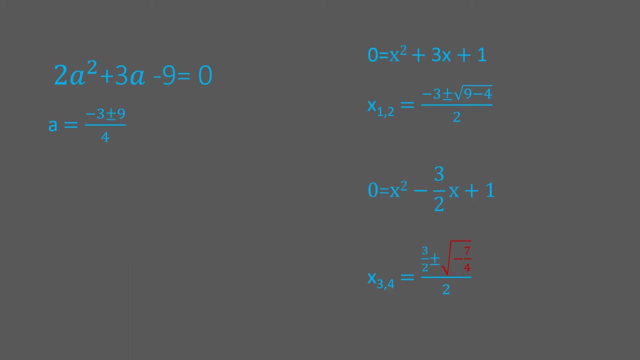 Stop That. discriminant is negative. So this equation don't give us any real solutions. Now we see that the equation has only two solutions. Here they are. In general, we can replace the coefficients by a, b and c to see that it doesn't matter. 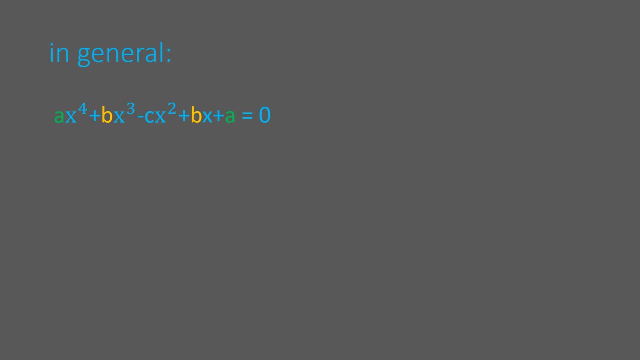 which numbers there are, As long as the coefficients are symmetric. So what are the pros and cons of this method? The first point is that you don't have to guess solutions and perform long division. The second point is that this method gets you solutions, no matter whether they are nice.